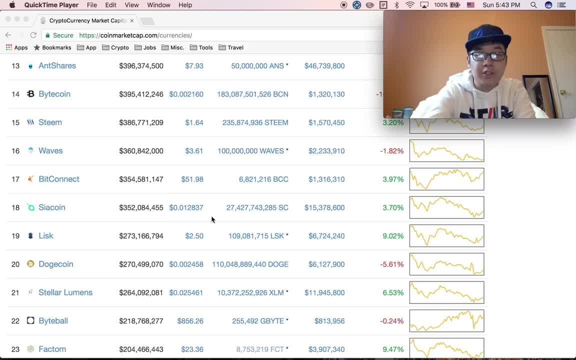 And on the other hand, you look at a coin like SiaCoin. each coin is worth a little bit more than a penny, but there's a lot more. There is Let's Let's see 27 billion coins out there. 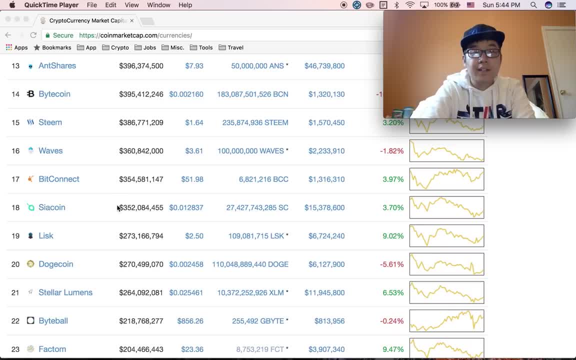 And so multiply those together, you get the market cap, And this can give you a way of more fairly comparing a coin's total value rather than looking at just the price, Because a lot of people out there on social media or other places they buy these cheap coins and they're like, oh, if this SiaCoin is worth each like $1,000 in the future. I'll be a multi-billionaire, But you can't really think about it that way, because the market cap is already kind of close, closer to Bitcoin's, And so if it's worth $1,000, it would be dwarfing Bitcoin's current valuation. 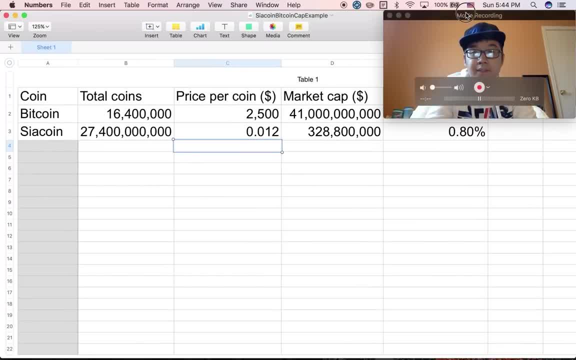 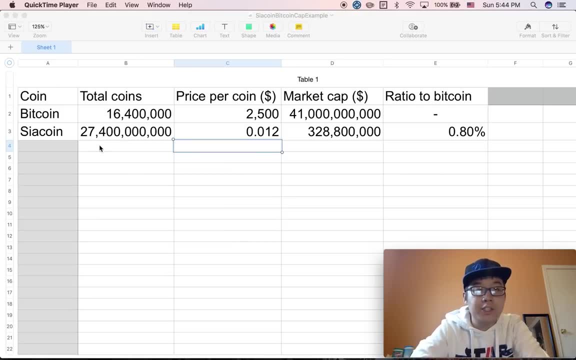 Let's take a look at the numbers for clarity. Let's move this down here. So this just shows us an example on a spreadsheet: Total number of coins, price per coin and market cap. And so right now, SiaCoin's market cap is 0.8% of Bitcoin's. 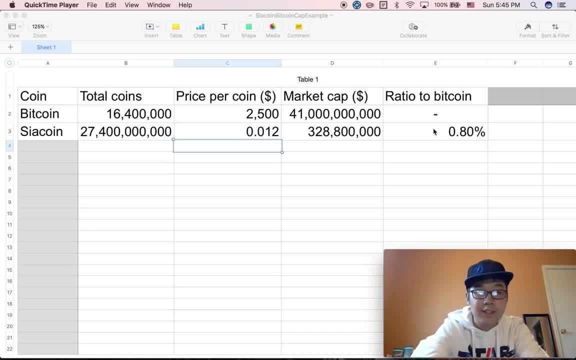 You can think about market cap as like total worth of this whole, all the coins collectively, And let's say it goes to $0.10 in the future. That would be 6% of Bitcoin's current valuation. Let's go up even further. 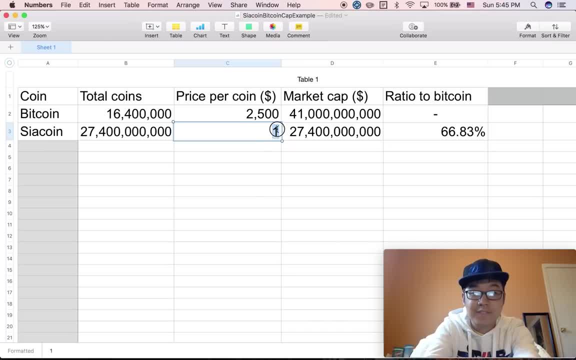 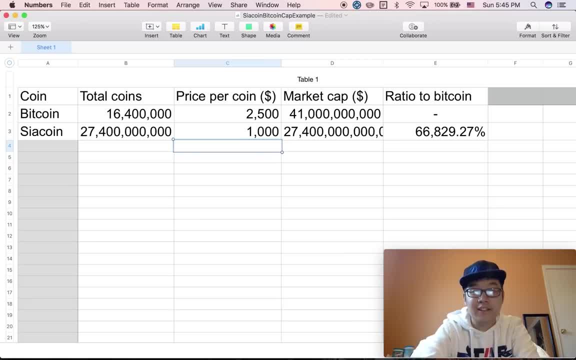 That would be 66,000% of Bitcoin's current valuation. Now, then, you have to ask yourself: do you think that's going to be the case ever in the future? I mean, it's possible, Nothing's impossible. Let's say, crypto blows up. 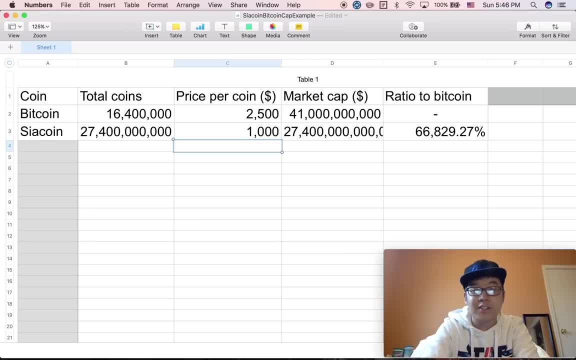 Like crazy And Bitcoin is worth trillions and trillions of dollars, And in that case, I guess it's not totally impossible for SiaCoin to be worth 66,000% of Bitcoin's current day 2017 total market cap.